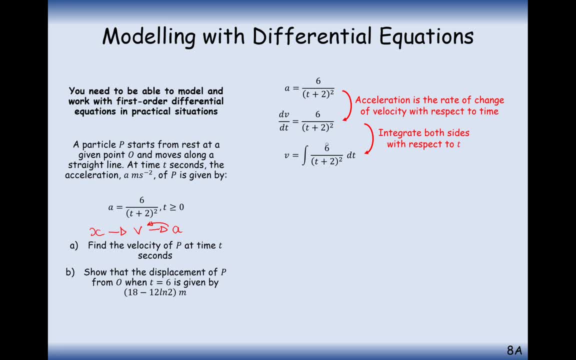 phi. And then you've got the integral of this expression here, And this expression here is going to be integrated by a little substitution. You may want to rewrite it as 6t to the plus 2 to the power of minus 2.. Use a substitution of something like: u equals t plus 2.. Then you'll. 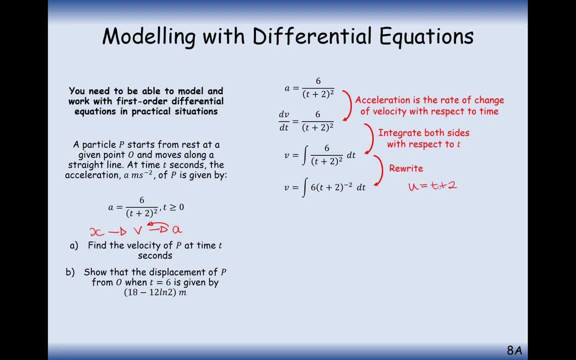 have to replace your dt with du. So just make sure you go through that whole process, But then integrate fundamentally And you'll get the answer. however you wish to do it, You may wish to do a kind of reverse chain rule on it, as 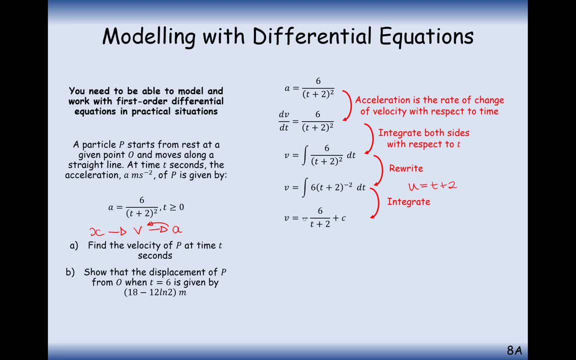 well, if you want to, But however you've done it, v is equal to minus 6 over t plus 2 plus c. So there we are. That's the answer for part a. Just to let you know, there's a mistake in the. 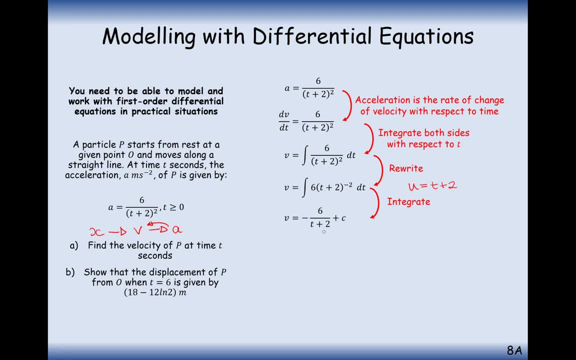 textbook at this point here I think they use a minus 2 inside the brackets there. This should actually be the question here: Find a velocity of p in terms of t seconds. I think we should be able to now find out what c is equal to, Because it says in the question here: from rest a given. 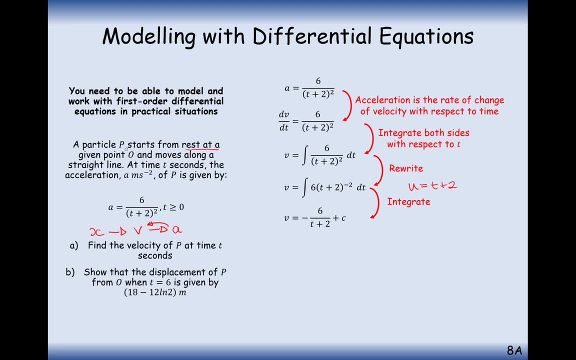 point t equals 0 starts, So it starts from rest, That's when t equals 0, v equals 0. So let's substitute that in, then t equals 0, v equals 0. And work out what c is equal to. So we've got 0. 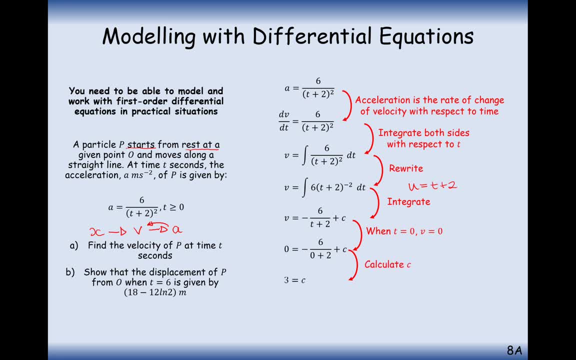 equals minus 6 over 2.. So that would be minus 3.. Move the 3 on to the other side And you get 3 equals c. Therefore, your final answer is v equals 0.. So that's the answer for part a of this question. 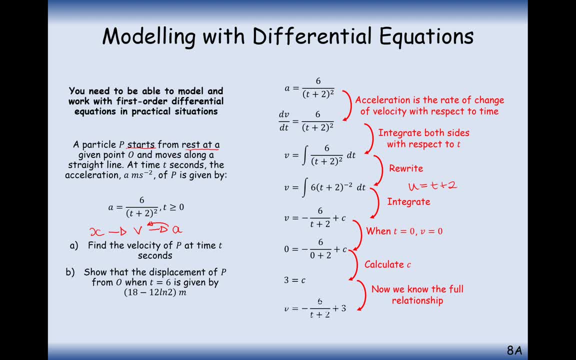 So that's the answer for part a of this question. So we'll see you next time. Bye-bye, Bye-bye, Bye-bye, Bye-bye, Bye-bye. So then it's going to be: v equals minus 6 over t, plus 2 plus 3 on the side. 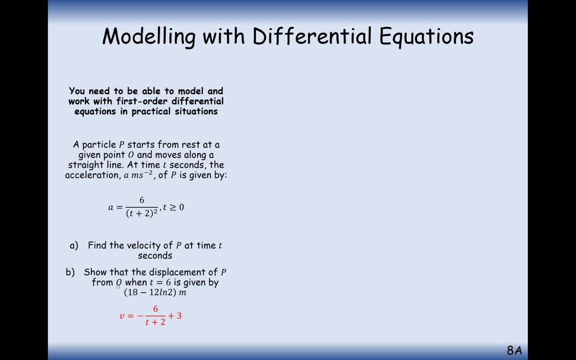 So that's our answer for part a. Now let's move on to part b. Show that the displacement of p from o when t equals 6 is given by this expression here. So we want displacement now. So that means we're going to need to integrate again to go from velocity to displacement. 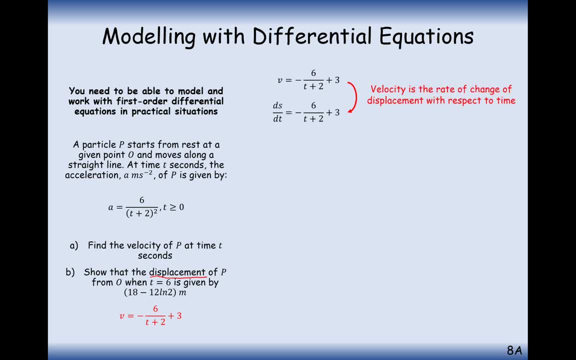 So again, let's integrate. So ds by dts is representing displacement here and is equal to what we have here. And now let's integrate with respect to dt. Now the first part of your integral here is going to be integrating by the Lund rule. 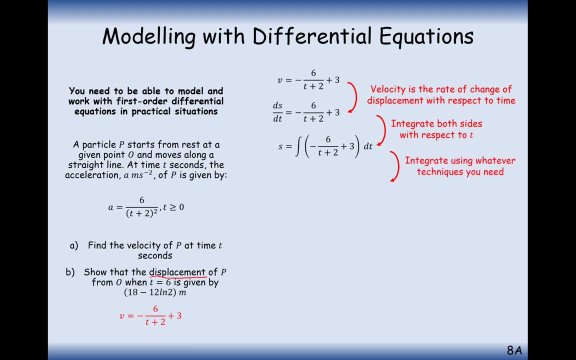 And then 3 will just integrate to 3t. So let's do that integration then. So it's going to be the Lund rule for this: minus 6 over t plus 2. 3 will integrate to 3t, And then we'll have. 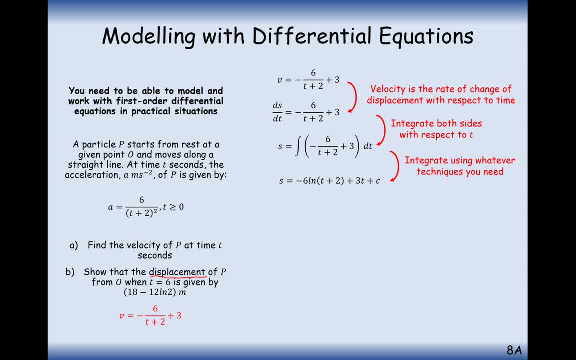 Plus c, And we need to show that when t equals 6, we get this expression here, But we need to work out what c is first. Now it starts from a given point: o. So in t equals 0, s equals 0. 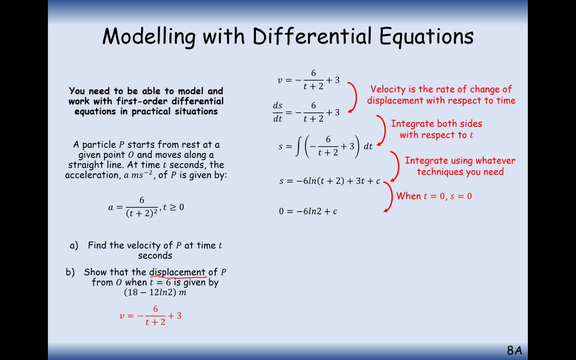 So substitute that in: It's going to be 0 here and 0 here, So it's going to be minus 6 Lund 2.. And then move that minus 6 Lund 2 onto the other side and you get 6 Lund 2.. 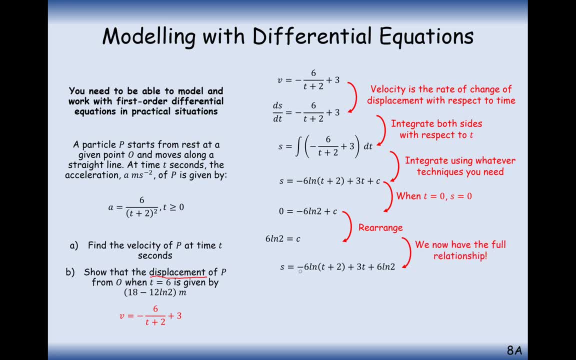 So your full relationship then Is: s equals minus 6 Lund t plus 2 plus 3t plus 6 Lund 2.. The final thing we need to now do with this is plug t equals 6 into this formula, So substituting t equals 6 then. 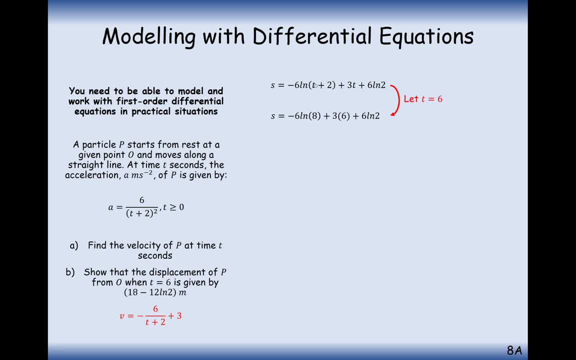 And we're going to get s equals minus 6 Lund 6 plus 2, which is 8 plus 3 times 6 plus 6 times Lund 2.. What we have to now do is simplify into this expression Here. now we're obviously we know where the 18 has come from, but now we need to simplify it all in terms of Lund 2.. 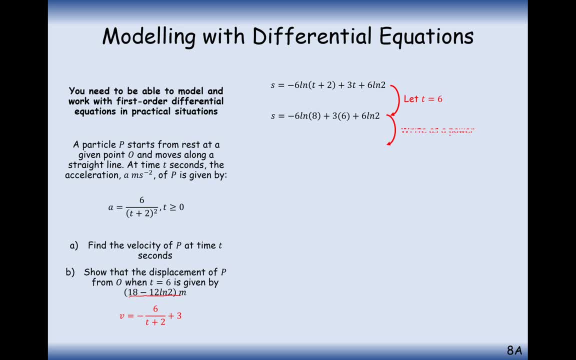 Recall the fact here that 8 is equal to 2 to the power of 3.. So it's 2 to the power of 3 here, And then we're going to move that power of 3 to the front as a multiplier. 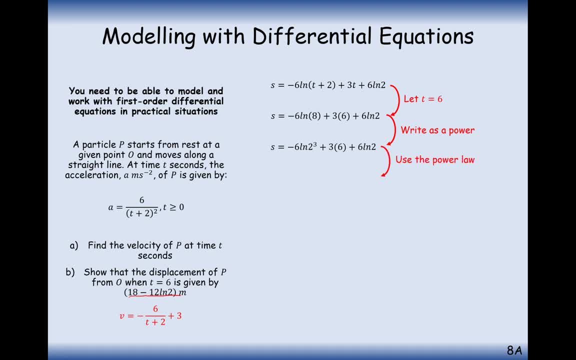 That's one of the rules of logs. So apply a rule of log to get the minus 18 Lund 2 at the start, But then group it together with this 6 Lund 2 at the back. So that's going to be minus. 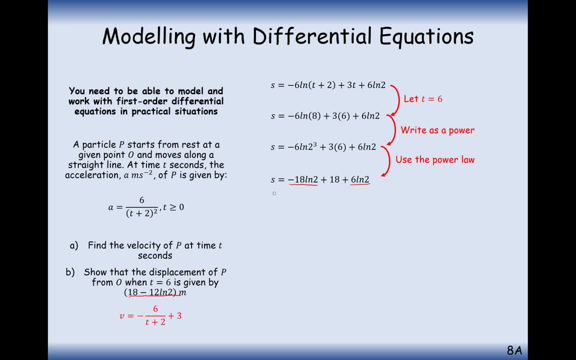 Minus 18 Lund 2 and 6 Lund 2.. And that's going to give you minus 12 Lund 2.. So it's going to be 18 minus 12 Lund 2 equals s, And that's going to be in meters. 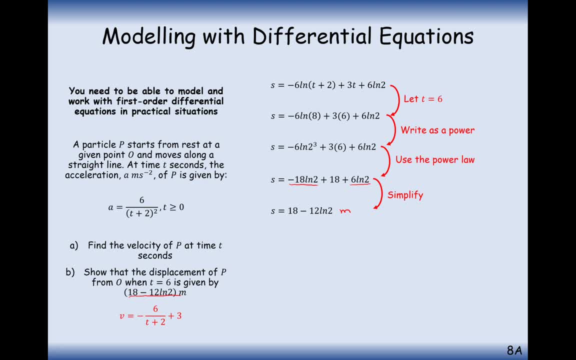 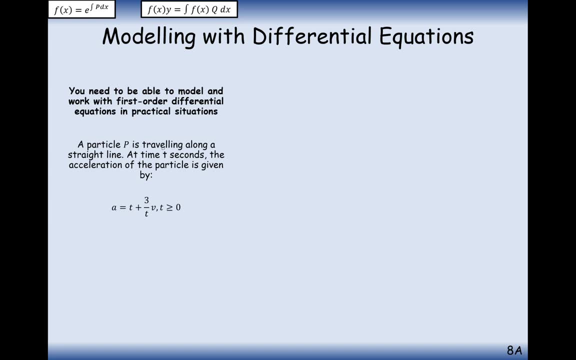 So there you are. That's the answer for part b, And that's the first question. fully complete, then. OK, so let's move on to the next question. A particle, p, is travelling along a straight line at time t seconds. The acceleration of a particle is given by this expression here: 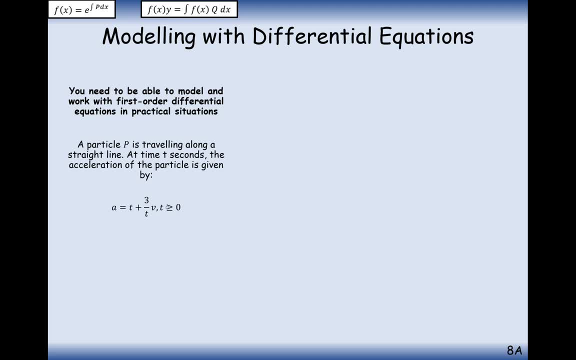 a equals t plus 3.. 3 over t v, where t is positive or equal to 0.. So our question is: given that v equals 0 when t equals 2, so that the velocity of the particle at time, t seconds, is given by the equation. 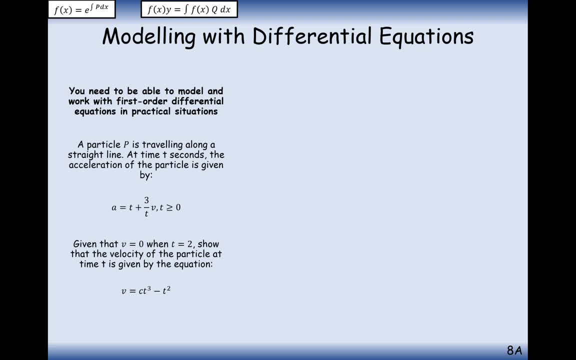 v equals ct cubed minus t squared. This one's a little bit more difficult to the one before because it's got a t and v in the formula, So we may need to use a more complicated strategy to solve this. So just a reminder: the first thing we need to do in a question like this: 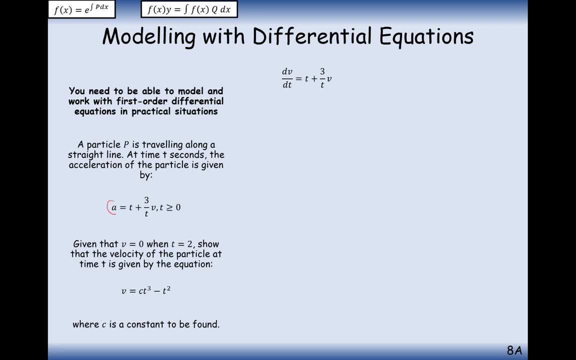 is convert some of the letters into each other, So a. if you remember me saying that a is velocity differentiated. well, that's the first thing I've done. I've replaced acceleration with velocity differentiated dv by dt, And then what I'm going to do is I'm going to move the 3 over t v onto the other side. 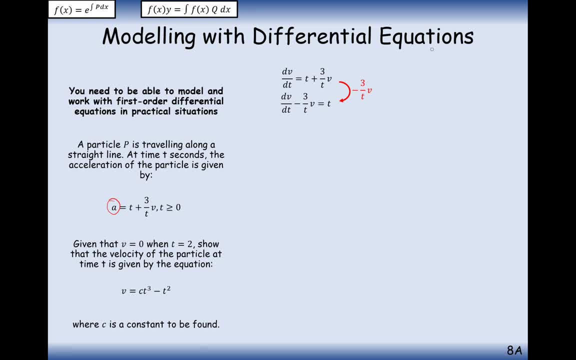 So now it looks a little bit like a first order differential equation. It looks a little bit like dy by dx plus py equals q, where y is representing v and x is representing t. There's some function of t in front of the v. 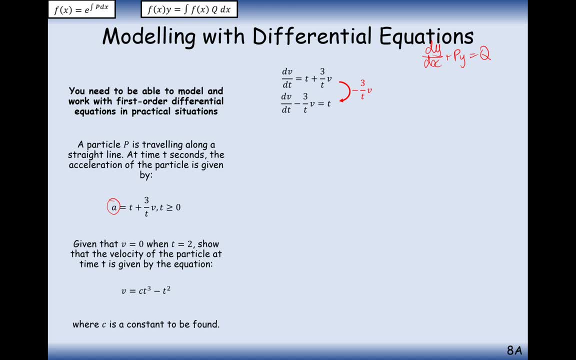 and then there's some function of t at the back. So it looks just like a first order differential equation. where we have this type of form And when it's of this type of form, the first thing we need to do is work out an integrating factor. 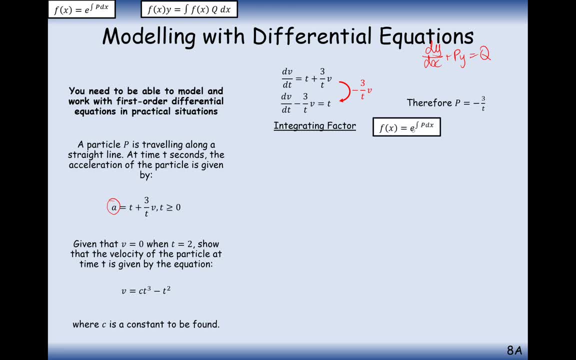 And the integrating factor is e to the integral of p, dx, where p is the coefficient of v. So p in this case is minus 3 over t, whatever's in front of v. So let's work that out then. 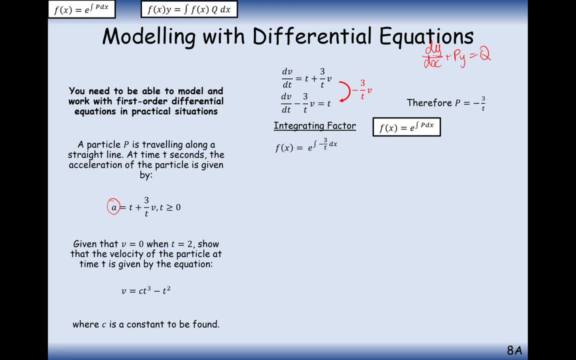 So it's going to be the integral of, say, e to the integral of minus 3 over t, dt. that should be Integrate it and we're going to get minus 3 ln, t, Then put the minus 3 inside the ln, using that rule of powers, and then cancel out. 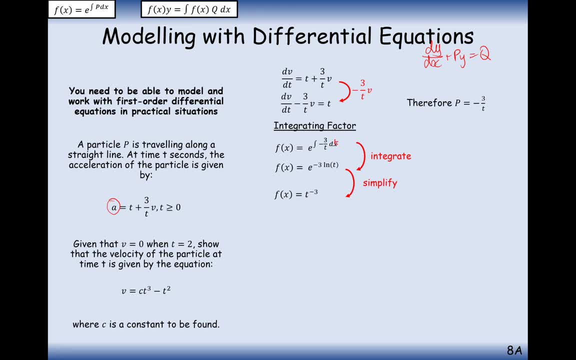 the e and the ln, And we get t to the minus 3.. So this is our integrating factor. This should all be f of t. Beg my pardon. OK, so now what we're doing. the second stage of a first order. 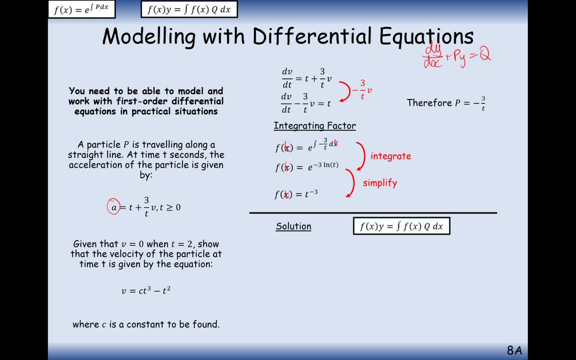 differential equation problem is to now start solving it. The solution is always of this form: here f of x- y equals integral of f of x, q, dx. However, we're not using the letters x and y here. We're using v and t. 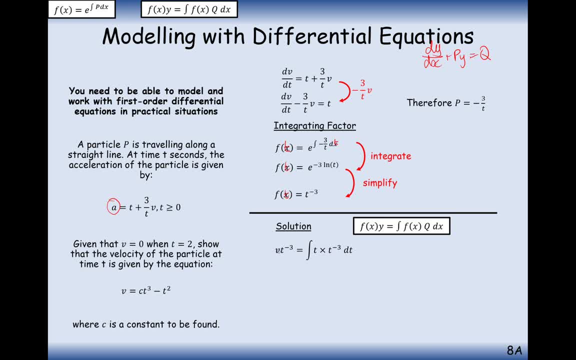 So it's going to be v, that's the y bit times t to the minus 3, that's the f of x bit. equals the integral of t, that's the q bit times t to the minus 3, that's again the f of x bit, dt. 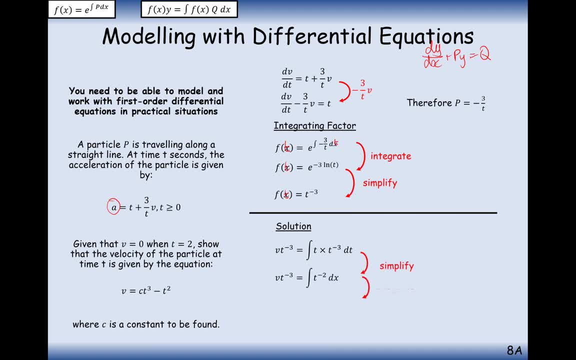 So let's now simplify what we've got there and now integrate, So we get minus t to the minus 1 plus c and then multiply by t, cubed on both sides. That will cancel out the t to the minus 3 on the left. 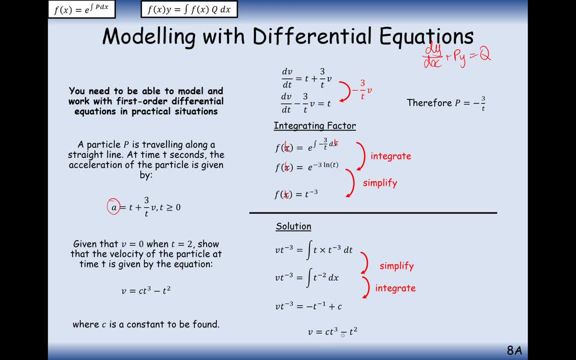 So we get v equals ct cubed minus t. OK, so the next bit we need to do then is: c is a constant to be found, OK, so we're also told here that v equals 0, t equals 2.. So let's plug that in and work out what c is. 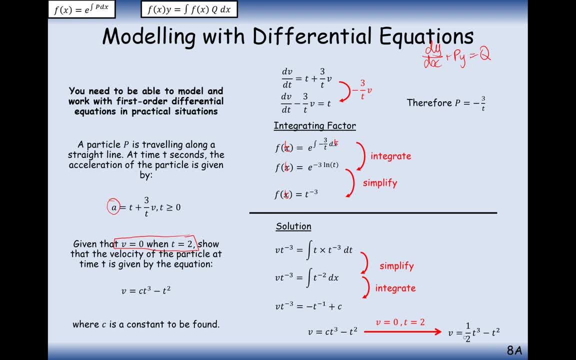 Then, once you've plugged in those two and worked out what c is, you work out that c is a half, So v equals a half t cubed minus t squared. And there we are. That's the answer to this question. OK, so moving on to the final question. it's a very long one, this one. 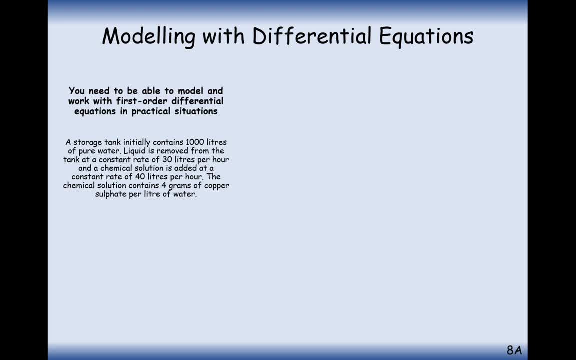 A storage tank initially contains 1000 liters of pure water. Liquid is removed from the tank at a constant rate of 30 liters per hour And a chemical solution is added at a constant rate of 40 liters per hour. The chemical solution contains 4 grams of copper sulfate per liter of water. 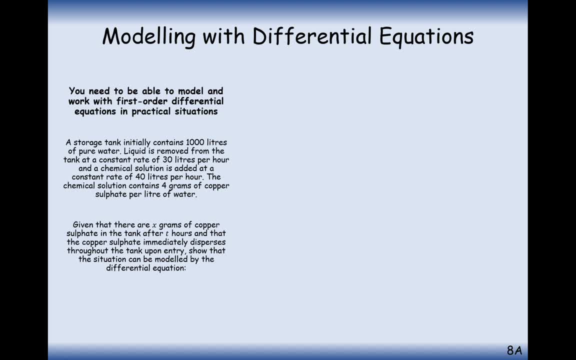 Given that there are x grams of copper sulfate in the tank after t hours and that the copper sulfate immediately disperses throughout the tank upon entry, show that the situation can be modelled by the differential equation, And it's going to be: dx by dt equals 100 minus 3x over 100 plus t. 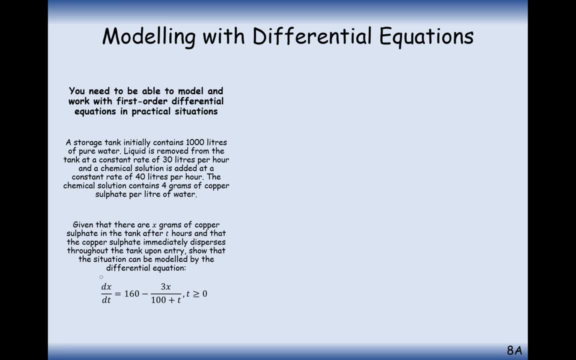 OK. so we need to work out where on earth all of these things have come from and give a good explanation as to how we convert this situation into this differential equation. So this is what we're looking to show: dx by dt here is representing. 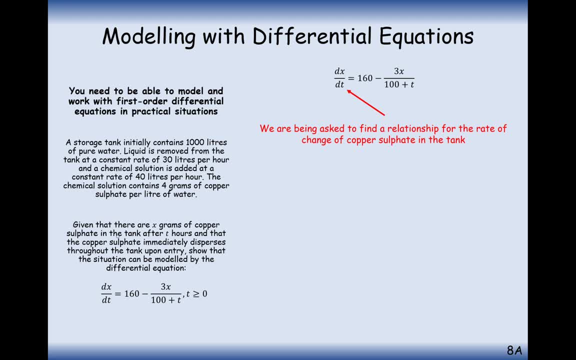 the rate of change of the amount of copper sulfate in the tank. every hour It's the rate at which that's changing by. So we're asked to find the relationship for the rate of change of copper sulfate in the tank. This would depend upon the amount of copper sulfate being added into the tank. 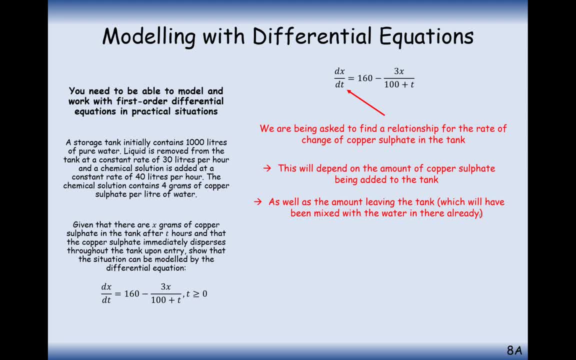 as well as the amounts leaving the tank, which will have been mixed into the water already. So if we imagine, after three hours there will already be some copper sulfate in the tank, But part of that will be leaving, because 40 liters leave the tank per hour. 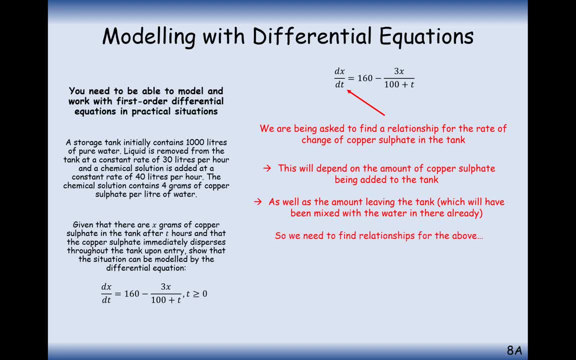 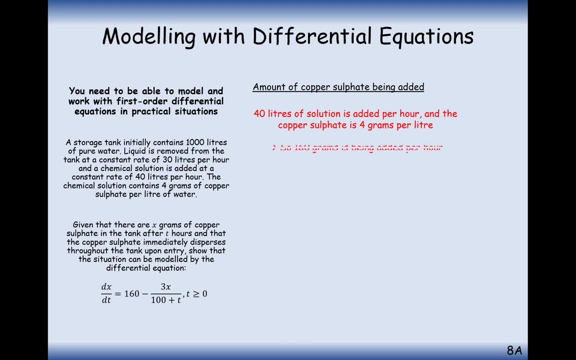 So that will include some of the copper sulfate. So we need to find the relationship for the above. OK, let's get started. The amount of copper sulfate being added: If we had 40 liters of solution per hour, then the copper sulfate is 4 grams per. 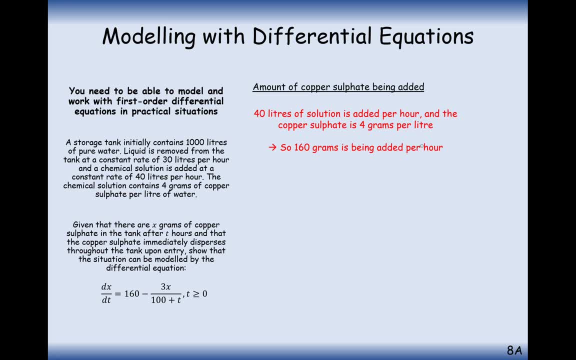 liter, then it's going to be 160 grams being added to the tank every hour. That doesn't mean that that will later on be affected by some leaving. Some of that 160 grams that was added in the first hour will leave in the second. 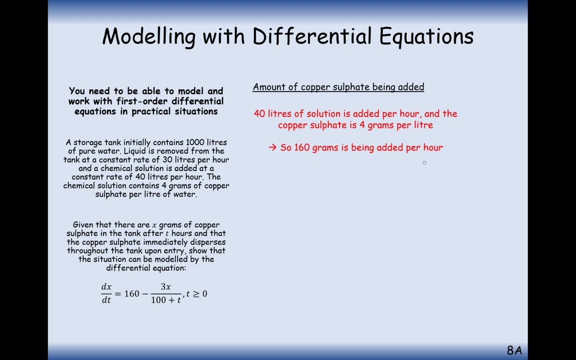 hour, but every hour at least, there will be 160 grams added to the tank per hour. So that's why we have 160 at the front of this equation. Now we need to think about this bit at the back here, which is representing: 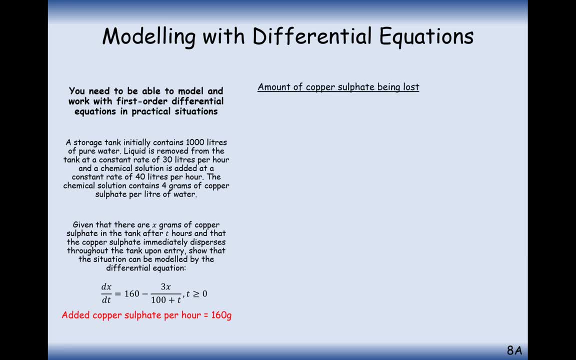 the amounts that leaves the tank every hour, So the amounts of copper sulfate being lost. We need to know What fraction of the liquid in the tank is made up of copper sulfate, So we need to know how much liquid is in the tank at any given time. 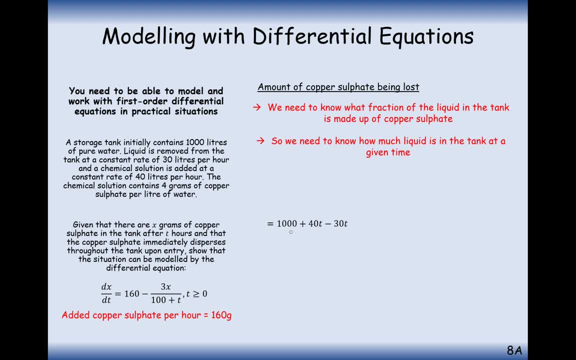 The amount of liquid in the tank at any given time starts with thousands, and then we add 40 liters per hour, so that'll be 40 times T. Then 30 leaves the tank every hour. So liquid is removed from the tank at a constant rate of 30, so it's removed at. 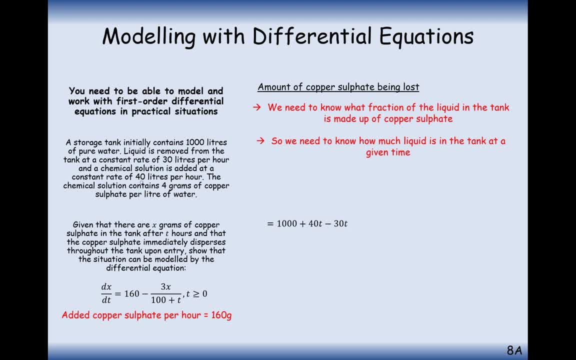 the constant rate of 30. So that's why it's a negative, and added at a rate of 40 liters per hour. So that's why it's 40 T as a positive. So this is the amount of solution being added and that's the amount of solution being removed. 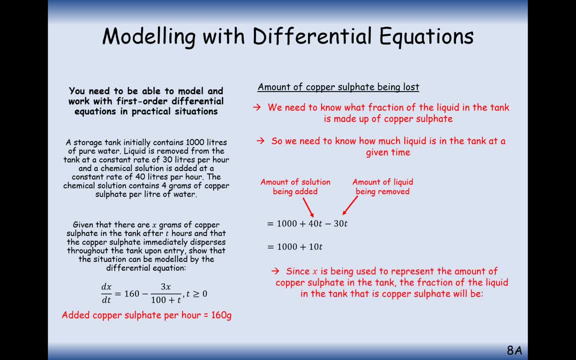 So simplifying that it's 1000 plus 10 T. And since X is being used to represent the amount of copper sulfate in the tank, the fraction of the liquid in the tank that is copper sulfate will be. so X is being used. 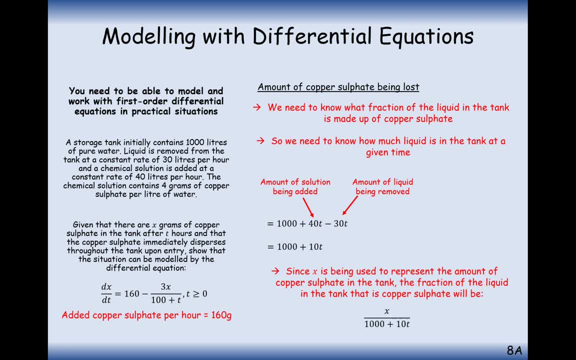 to represent the amount of copper sulfate in the tank. So it's going to be that fraction X being the amount of copper sulfate in the tank divided by 1000 plus 10 T. So how do we get the three on the top there? 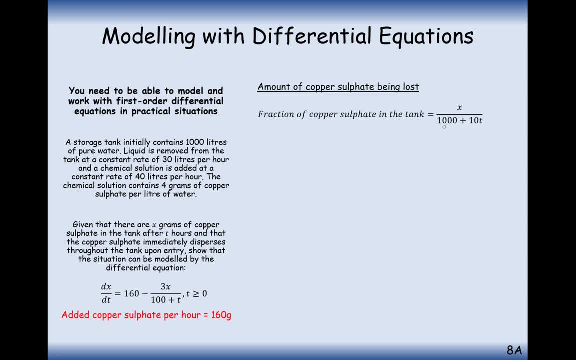 So the fraction of copper sulfate in the tank is X over 1000 plus 10 T because X if we go back down here, given that there are X grams of copper sulfate in the tank after T hours. so we know that if we say at five hours, we know there are X. 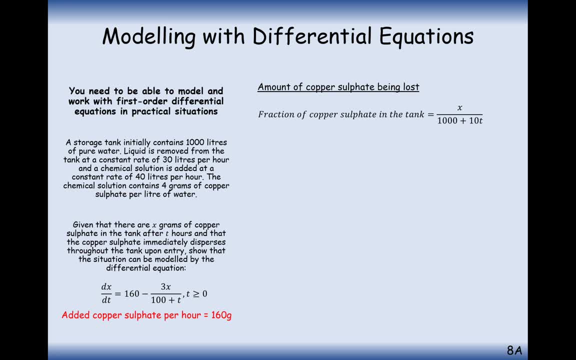 X. that's a letter that will change. X will be the amount of copper sulfate in the tank after that many hours. OK, so X over 1000 plus 10 T is the fraction of copper sulfate in the tank. So the bottom of this fraction is how much liquid is in the tank. 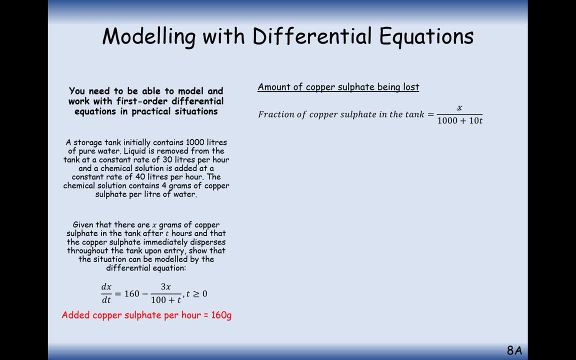 And X is the amount of copper sulfate in the tank. But given that we have 30 liters of liquid in the tank, that leaves every hour, some of which contains that copper sulfate, So we need to multiply the fraction by 30 to give the amount of. 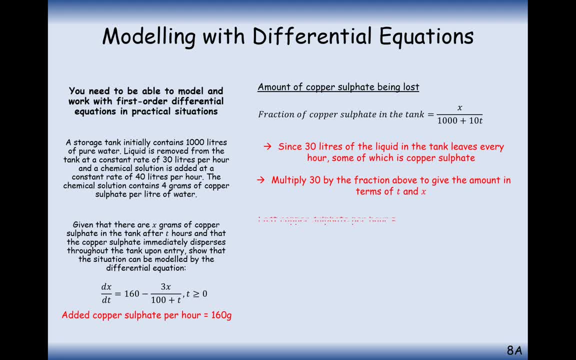 to give the amount in terms of T and X. So the amount of copper sulfate that's lost every hour is the fraction of copper sulfate that's in the tank times 30 liters every hour. So when we multiply those two fractions together, times the factor of 10 on the top. 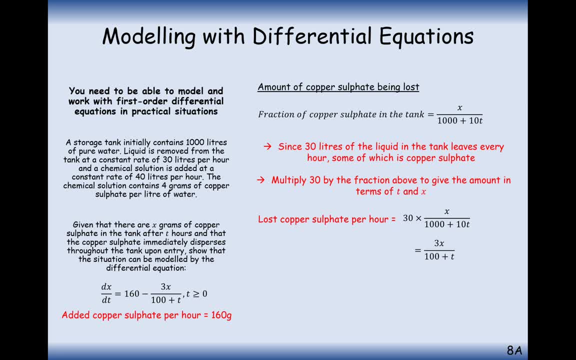 and bottom. so cancel out a factor of 10 on the top and bottom and we have 3X over 100 plus T. So what we calculated here is the amount of copper sulfate lost per hour, which is the fraction of copper sulfate that's in the tank times. how much we want. 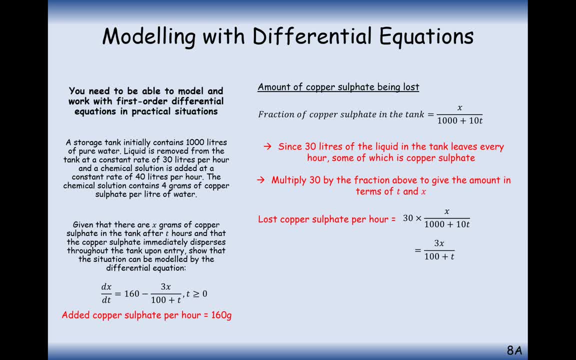 to leave in the tank. so that would be 30 as a multiplier. So the amount of copper sulfate added per hour is 160 grams. The amount of lost copper sulfate per hour is 3X over 100 plus T. So there we are. 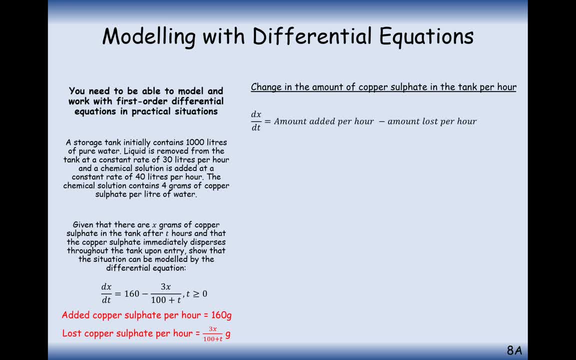 So in the differential equation the change in the amount of copper sulfate in the tank per hour is: DX by DT equals the amount added. take away the amounts lost per hour. So it's going to be 160 minus 3T over 100 plus T. 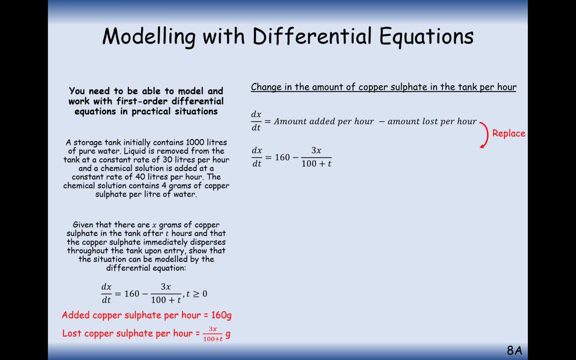 And these questions here are actually becoming more popular in the further maths exam at the moment, So make sure that you've understood this. maybe go back and rewatch it again, But then have a go at these types of questions in exercise 8A please. 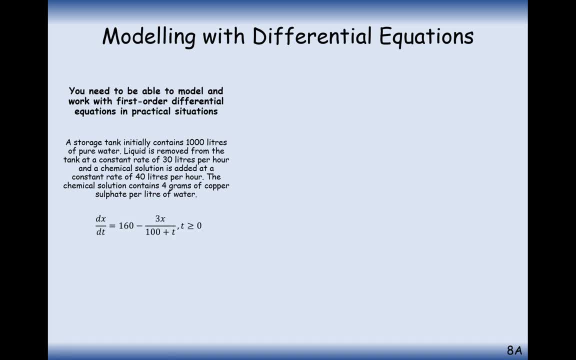 OK. so amounts added, take away the amounts lost. OK. so now that we've got the equation, let's go ahead and solve the equation. So the question here is: find the number of grams of copper sulfate in the tank after six hours. 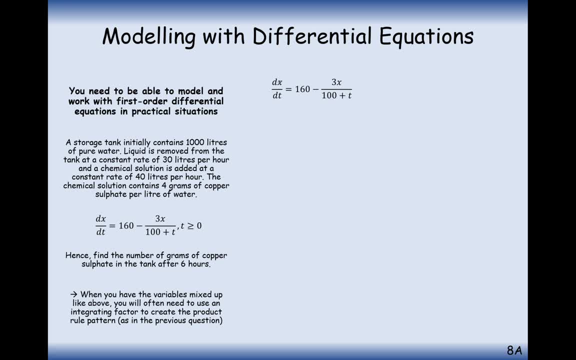 So the differential looks like this: It's DX by DT equals 160 minus 3X over 100 plus X. We could move all the T's onto one side or the X's onto another and then solve the derivative that way. It doesn't look like you'll be able to do that. 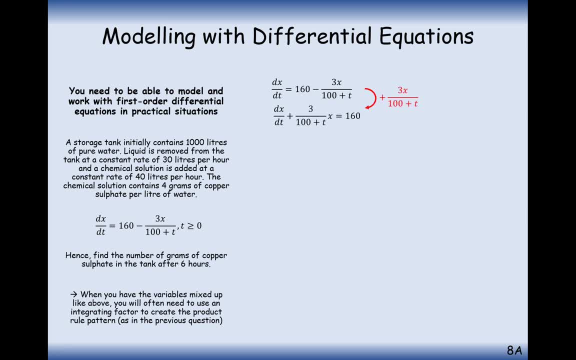 What we'll have to do here is move the 3X over 100 plus T onto the other side and then solve it like we would. a DY by DX plus PY equals Q derivative, where we need to use an integrating factor and P is the function that's in front of the independent. 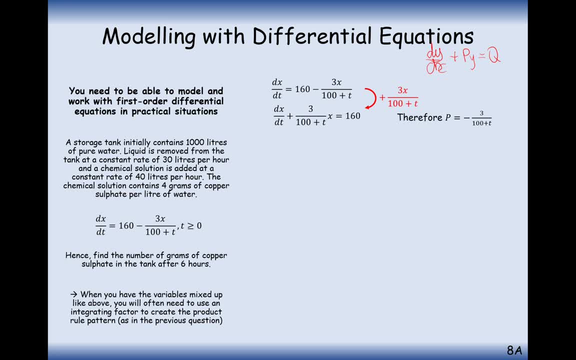 the dependent variable. So P is therefore positive 3 over 100 plus T. Let's now work out what the integrating factor is going to be. Integrating factor is always of the form E to the integral, PDX or T, depending on what your independent variable is. 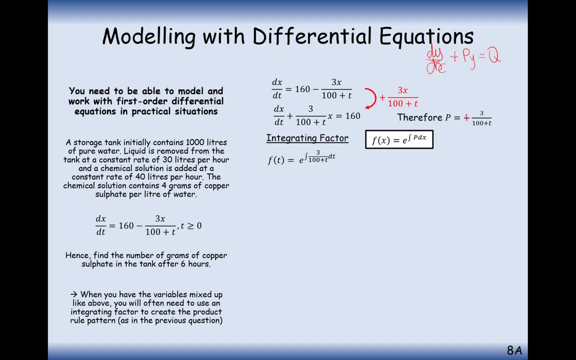 So E to the integral of 3 over 100 plus T DT. Let's now integrate that power, So that's going to be 3 LUN 100 plus T, Move the 3 in as a power on the LUN and then cancel out the E and the LUN. 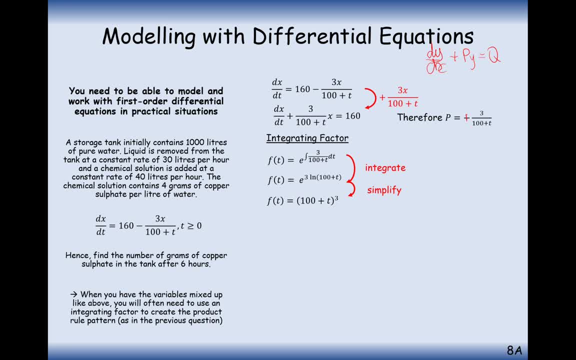 And we'll get F of T is 100 plus T all cubed. So without the integrating factor, we can now go for the solution, And the solution is always of this form: The integrating factor times Y- or in this case it's going to be X- equals the integral of the integrating factor times Q. 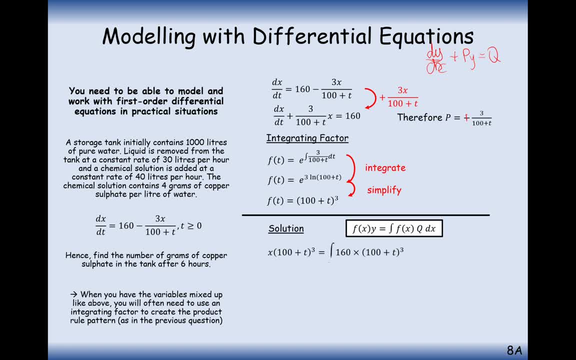 And that's the function on the other side of the integral. So this is what the next stage looks like. It's going to be X times 100 plus T. all cubed equals the integral of 160 times 100 plus T cubed DT. 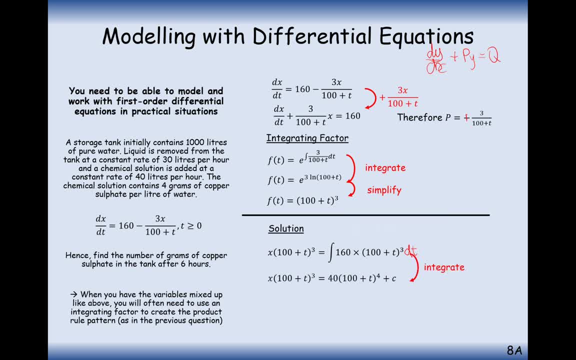 Next thing we'll need to do then is we'll need to integrate the right hand side. You could use a substitution of U equals 100 plus T if you wish to do so. That will lead you to 40, because you need to divide by four on the 160, and then you increase power by one. 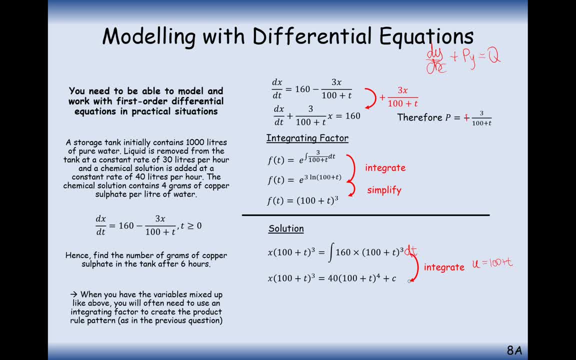 So it's 100 plus T to the power of four plus C. And if we were to then cancel out the 100 plus T's cubed on the left hand side, we'll be left with this: X equals 40 times 100 plus T plus C. 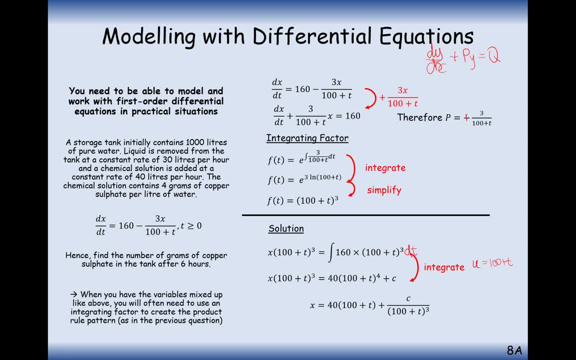 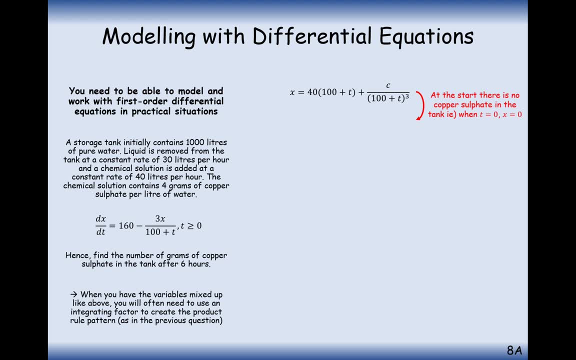 So that's C over 100 plus T cubed. So What we're told in the question is: initially there's no copper sulfate in the tank, So at time T equals zero, X equals zero. So let's plug that in and work out what C is. and C is going to be minus four billion. 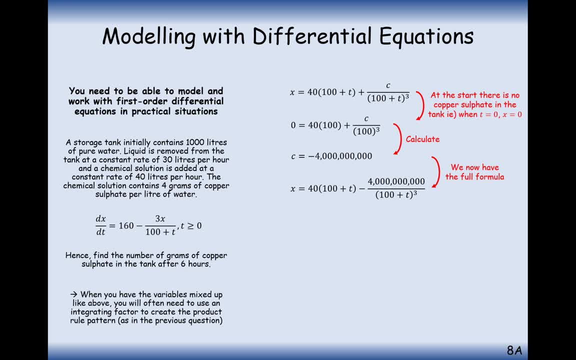 So minus four billion is the value for C. Never had such a big value of C before, And now we need to just plug in the value for T, equals six, to find out what X is, And do the calculations: 882 grams. So there we are. 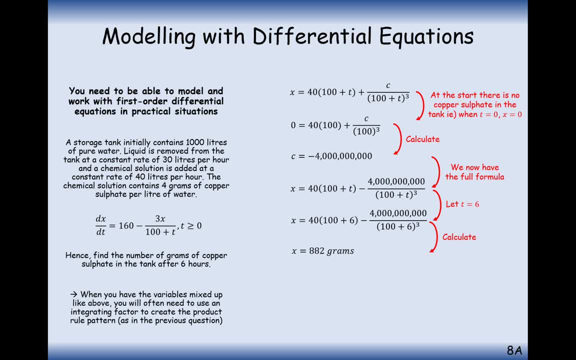 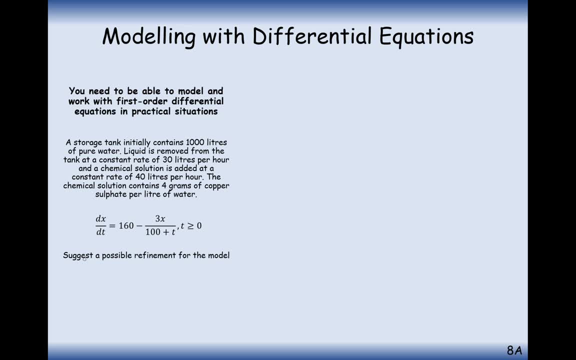 That's how many grams of copper sulfate are in the tank after six hours. Right, and move on to the final part. quick part here: suggest a possible refinement for the model. The model could be refined so that the copper sulfate does not immediately. 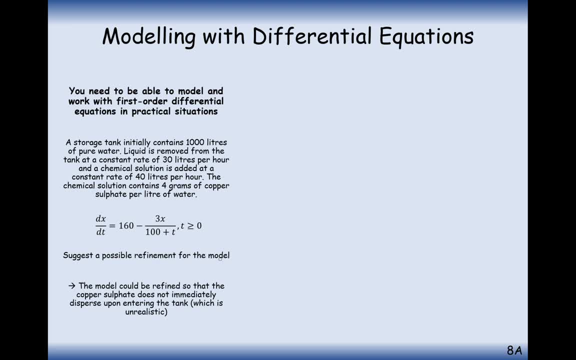 disperse upon entering the tank, which is unrealistic. Generally, the copper sulfate would cluster in certain areas Rather than disperse throughout the tank uniformly, because when it comes out of the tank it's going to come out uniformly while it's to do with the coming out of the tank. 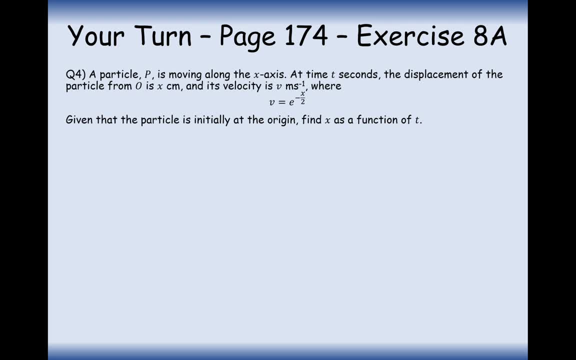 OK, let's move on to a question for you to have a go at then. This is question four from page 174.. Pause the video and give this question a go. OK, so let's have a go at question four then. A particle P is moving along the X axis. 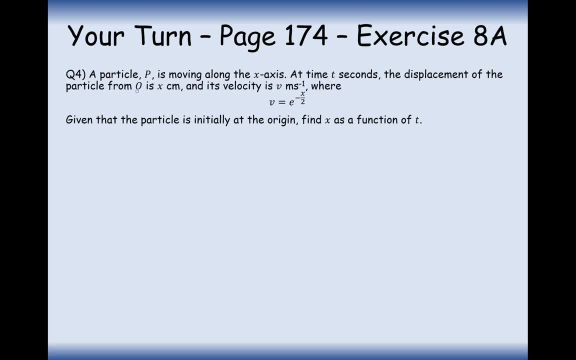 At time, T seconds. the displacement of the particle from O is X centimetres and its velocity is V metres per second, where V equals E to the minus X over 2.. Given that the particle is initially at the origin, find X as a function of T. 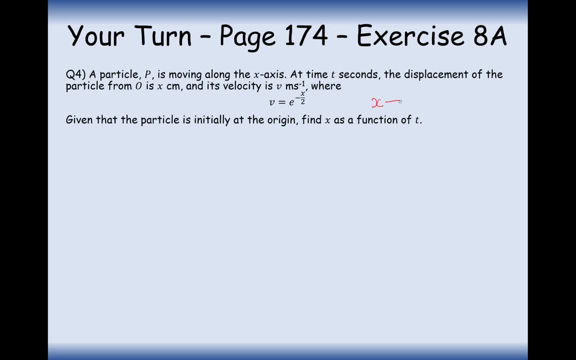 So the first thing we need to consider is that when you differentiate X, you get V. When you differentiate V, you get A. We don't need the second bit, but the first bit's important, because V is X differentiated. So it's going to be: 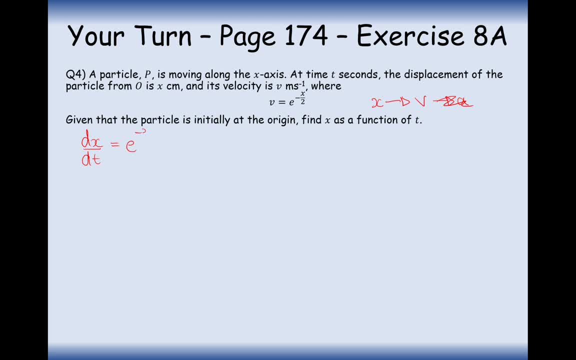 X by DT equals E to the minus X over 2.. Now it's a first order differential equation, but it's not the one where P and Q are involved, where we have to do an integrating factor. It's one where we just have to move everything onto the correct side. 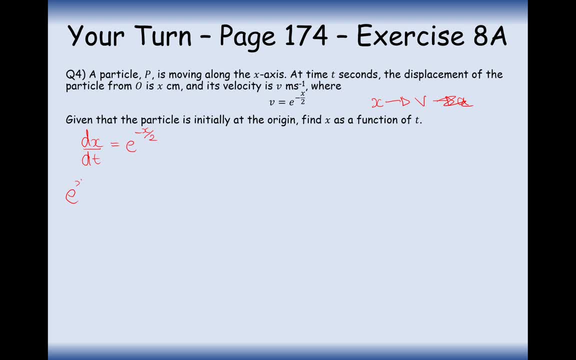 and then integrate it correctly. So I'm going to multiply by E to the X over 2 onto the left hand side, leave the X where it is and multiply by DT up onto the right hand side, effectively leaving behind a 1.. 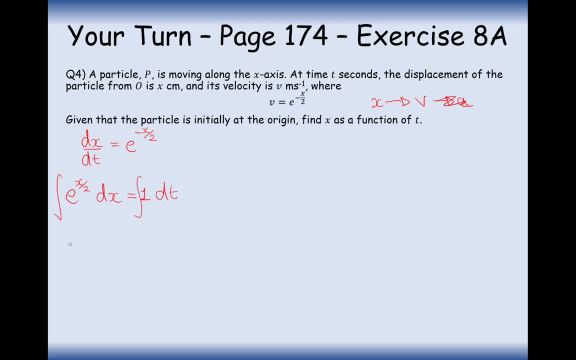 Then we can integrate both sides just like that. And then on the left hand side it's going to be 2 E to the X over 2 equals T plus C. Now, at this point I'm going to work out C, because it looks simpler. 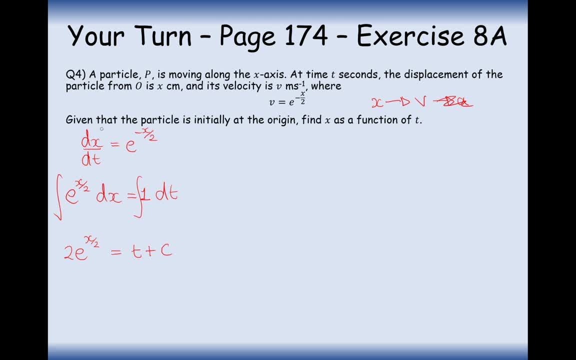 And then I'll rearrange it to get X equals. So it says: given that the particle initially is at the origin. So that means when T equals 0, X equals 0. So set X equal to 0, that's going to make it E to the 0,. 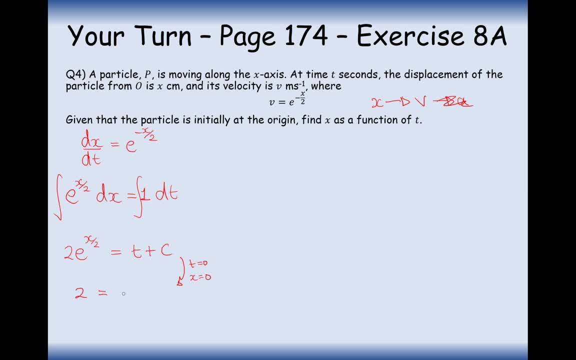 which is 1 times it by 2, you get 2.. So T is 0,. so C equals 2.. So this is going to equal then 2. E to the X over 2 equals T plus 2.. And now we have to rearrange this to make it X the subject. 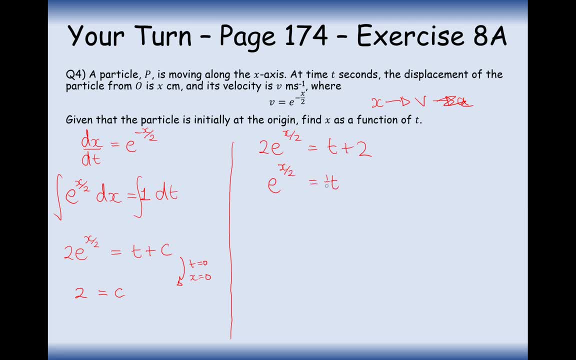 So divide both sides by 2, so it would be half T plus 1.. Then we get rid of the E by learning both sides. So X over 2 equals half T plus 1, and then times everything by 2.. So it's going to be X equals 2. learn half T plus 1..